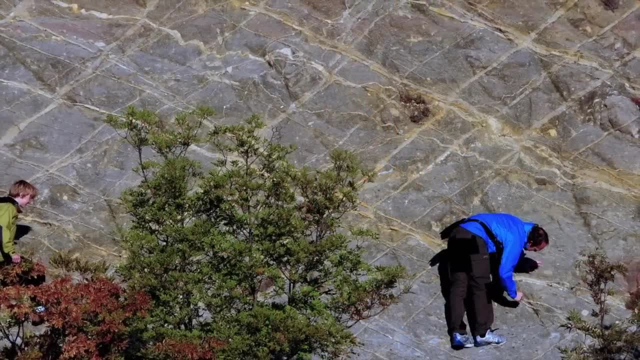 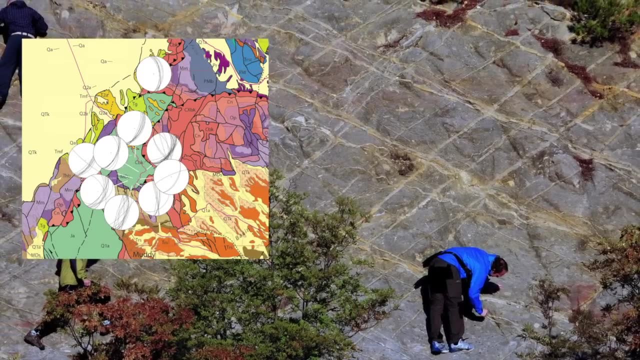 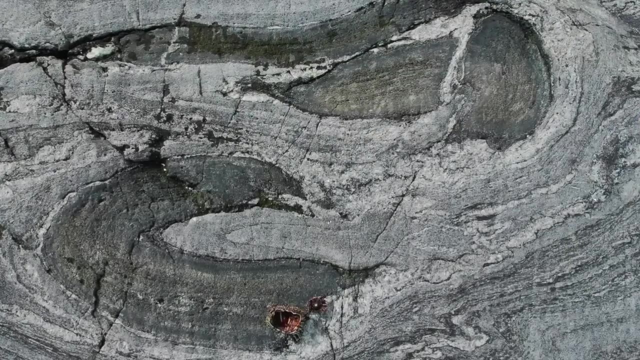 in the field and you can map them, you can measure up the orientations, geometries, go back and plot the data in stereonets and things like that, And that's a lot of fun, it's important, but it doesn't stop there. The most important part is to use the structural 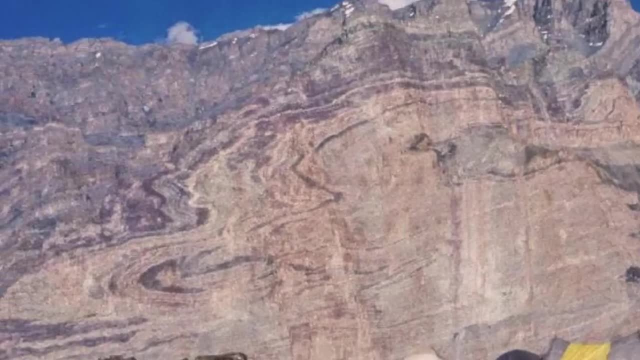 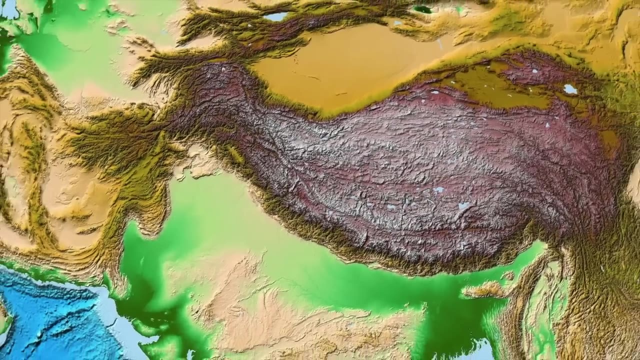 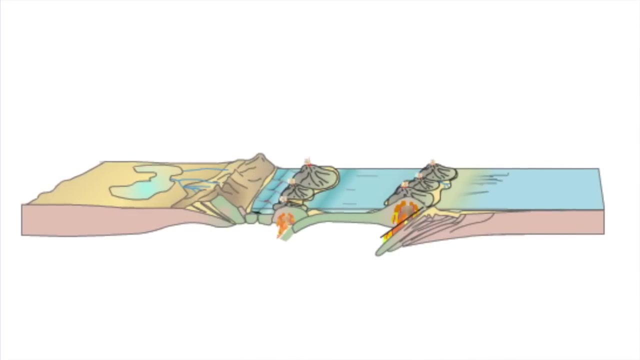 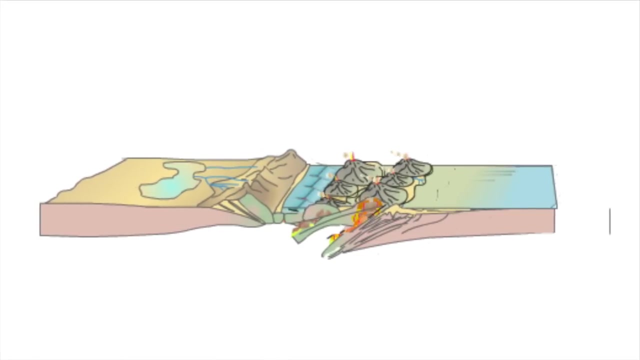 information to try and understand what's going on on a larger scale, And that's why structural geology is very closely linked with tectonics, including plate tectonics, where the motions in the crust, in the lithosphere, the motion of plates, is what creates structures. 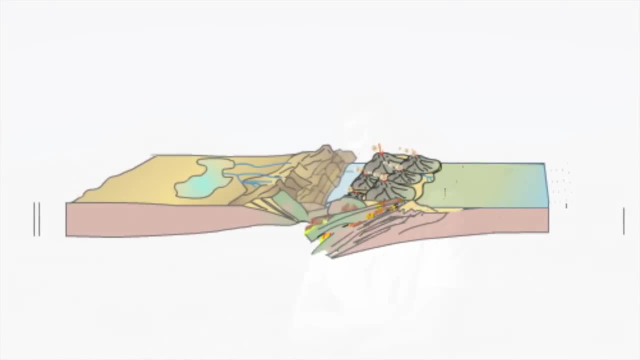 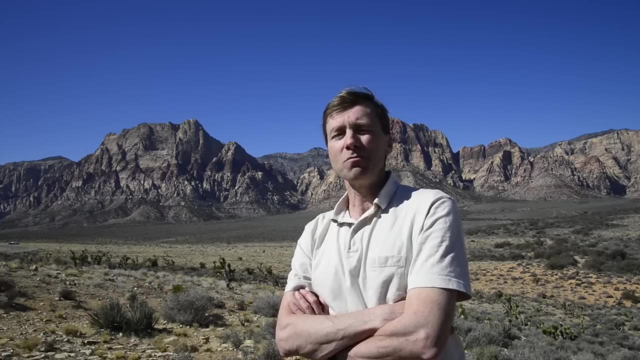 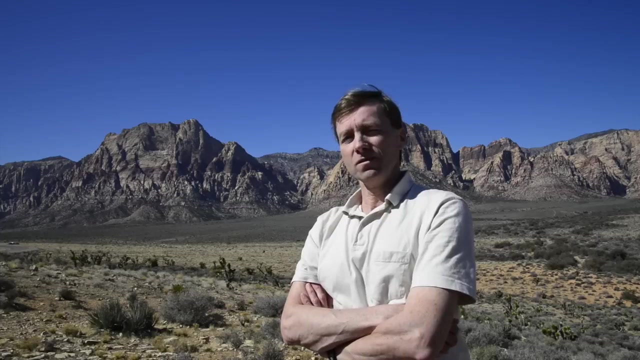 So we can use structures. if we know what we're looking at, if we understand how the structure is formed, We can use that information and try and say something about, for example, plate motions in the past As an example. we can take faults And there are different types of faults For 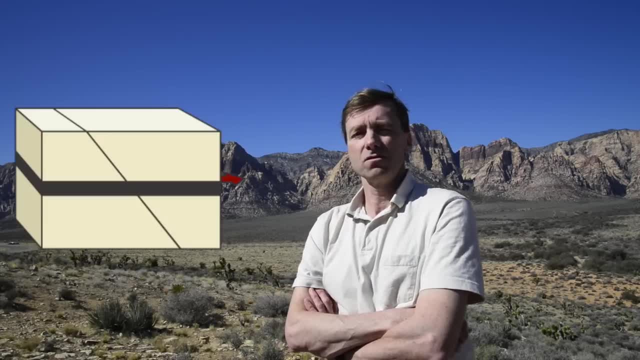 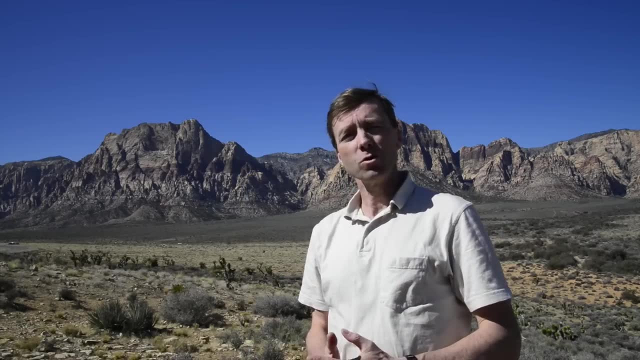 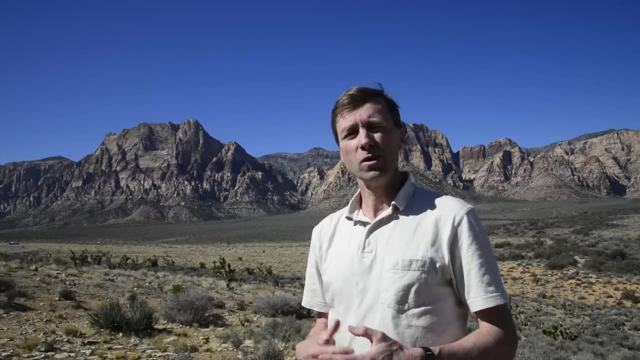 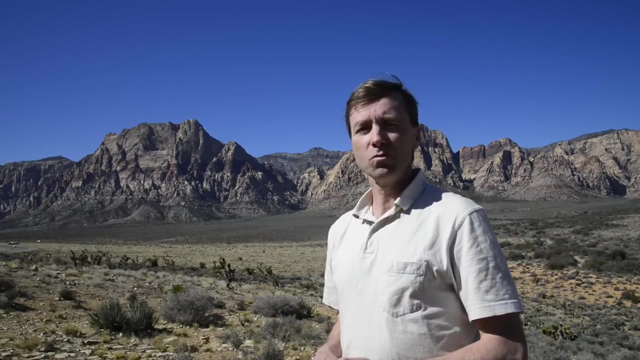 example, there are extensional faults, normal faults that are involved during the extension and stretching of the crust, And there are reverse faults and thrust faults that form is being shortened. Right now we are just outside of Las Vegas in the Red Rock Canyon area. We're looking at some red and yellow sandstones in the background. 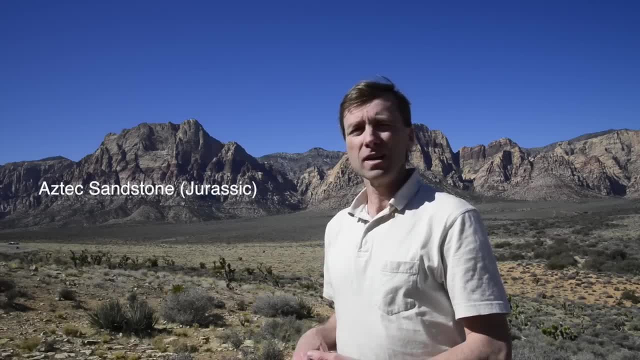 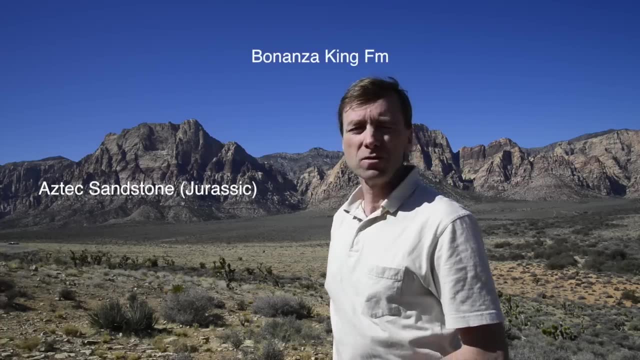 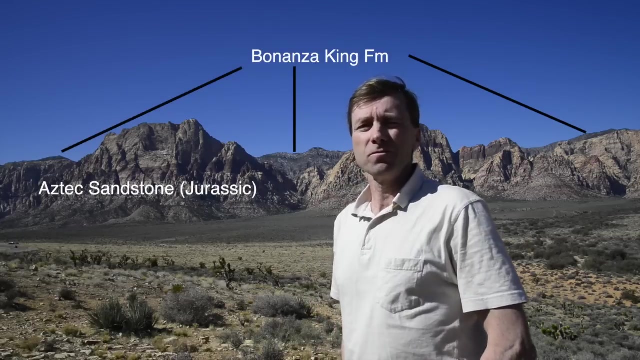 That's Jurassic sandstone, the Jurassic Aztec Formation. On top of those sandstones, back there in the mountain, there is another type of rock, another rocky unit that is older, That is Cambrian and Devonian, and those rocks, those old rocks, are resting on top of the relatively younger rocks. the 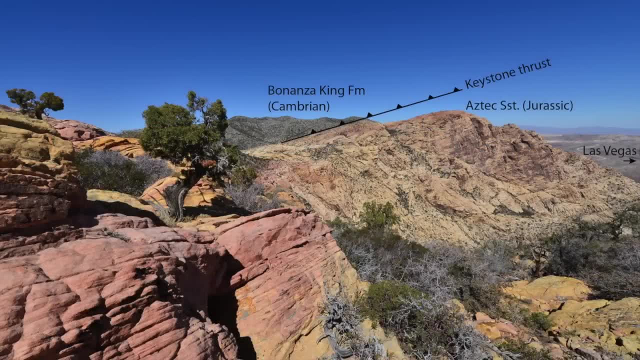 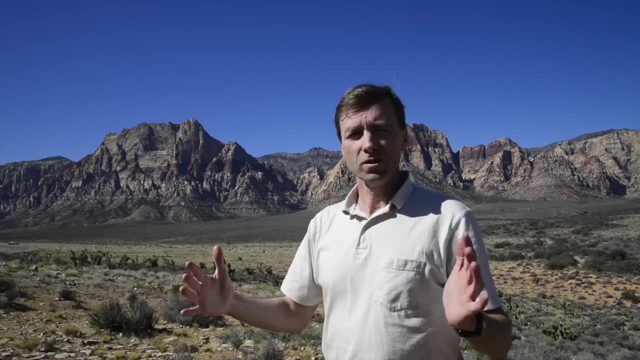 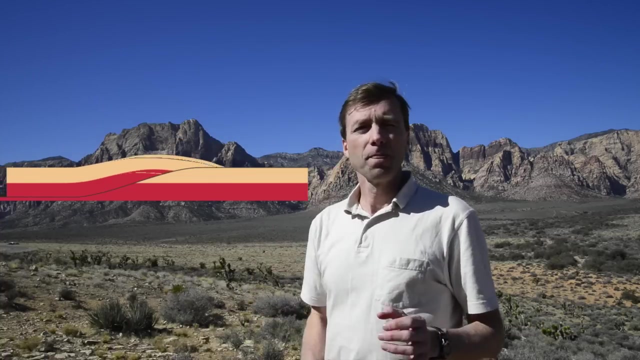 Jurassic rocks, So Cambrian rocks on Jurassic rocks. Between those units there is what's called a thrust fault, So that thrust fault formed between the two rocks When the part of the crust during shortening was ripped off and put on top of another part of the crust. So you get older rocks on top of younger rocks. 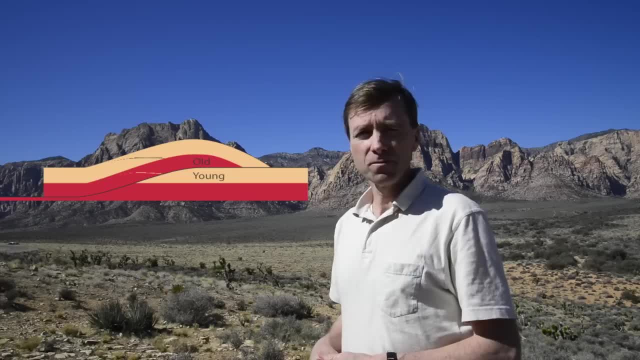 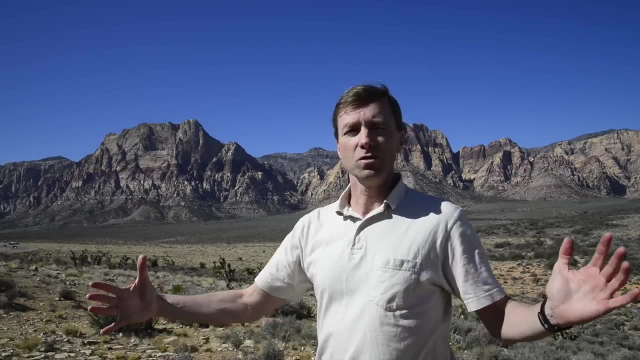 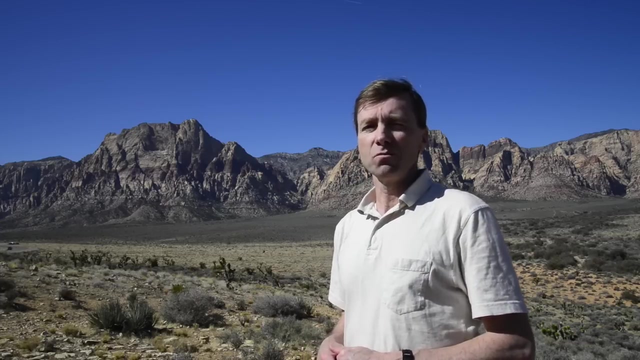 So that's one of the characteristics of thrust faults. Just understanding that relationship enables you to say something about the size and the magnitude of the shortening of this part of the United States, Sometimes after the Jurassic, probably in the Cretaceous, and this is actually the Sevier Orogeny and that particular thrust that 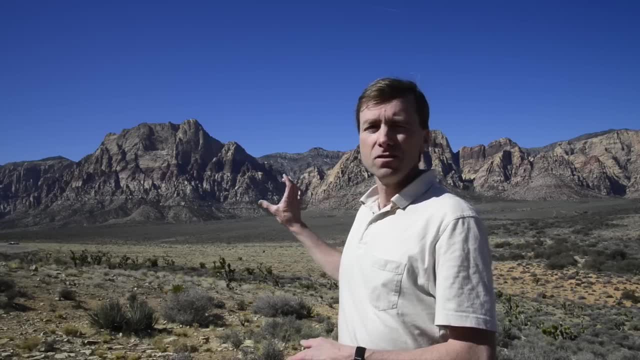 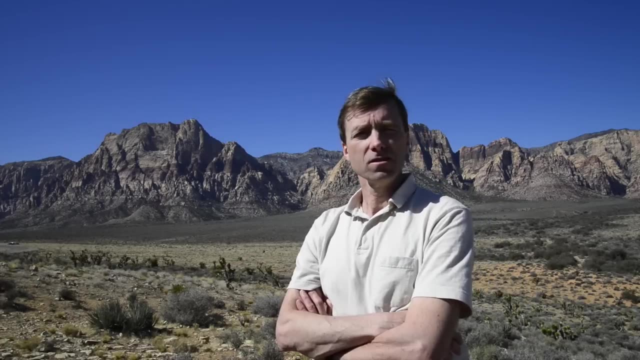 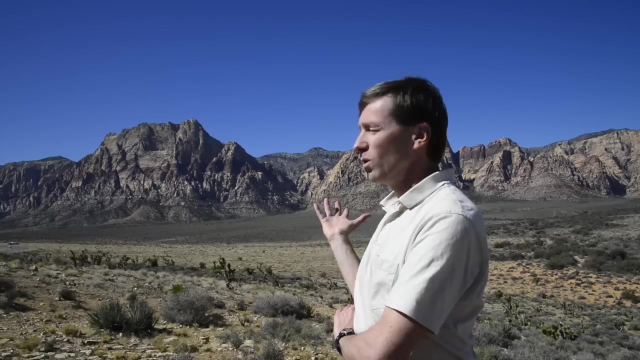 separates the upper plate. the Cambrian from the Jurassic is called the Keystone thrust in this area. Let's have a look at the plaster experiment, where we produce reverse faults and thrust faults, A little bit like what we have here in Red Rock Canyon outside Las Vegas. 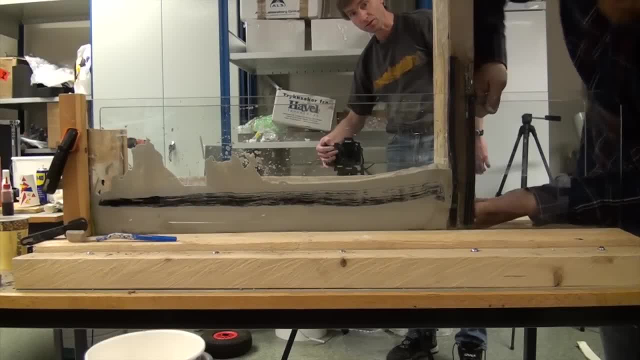 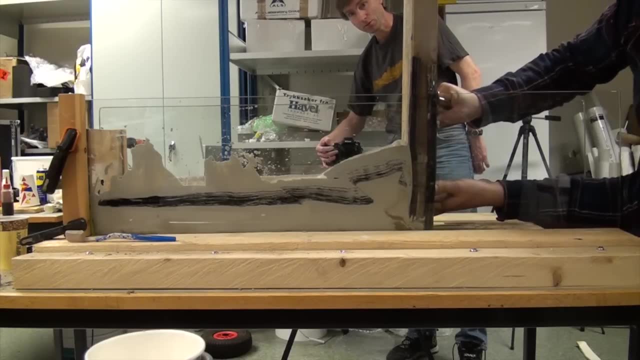 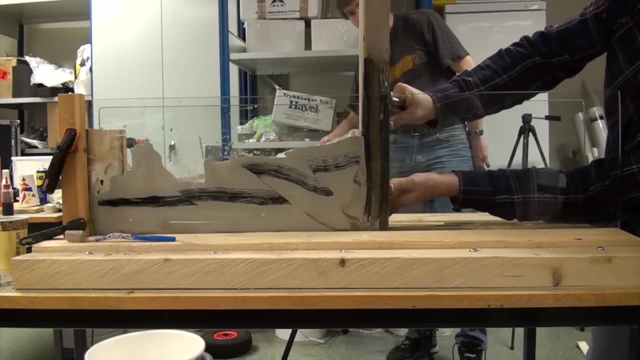 Well, this is an experiment where we are shortening wet plaster in a box, Shortening by pushing one side toward the other, and the nice thing about experiments is that we can see not only the end result, but we can see the entire development, from the beginning to the end, And in this case, we can see which of 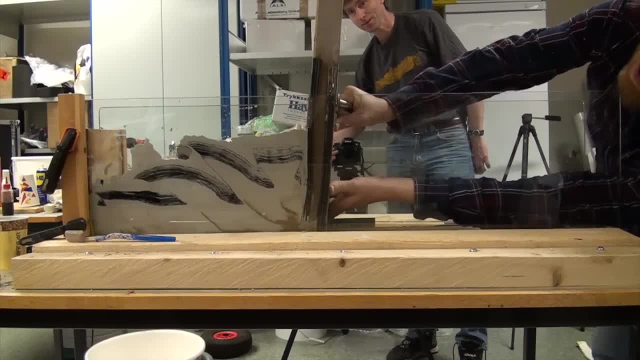 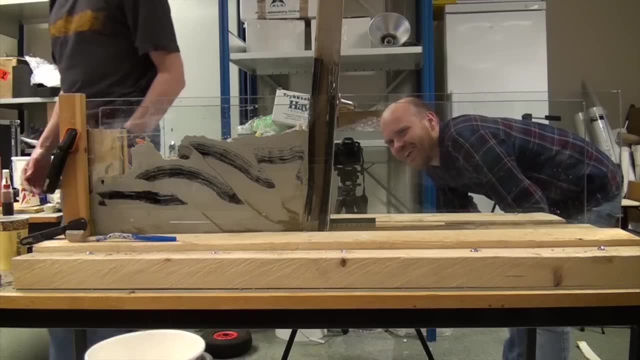 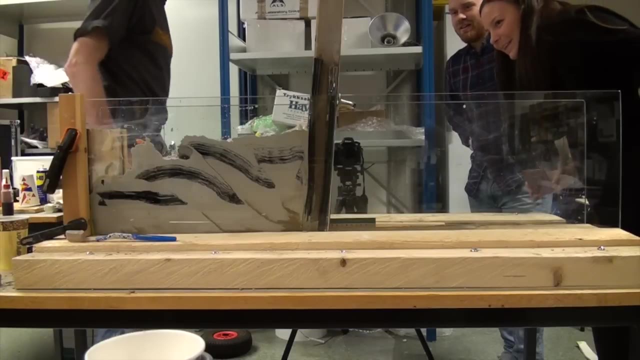 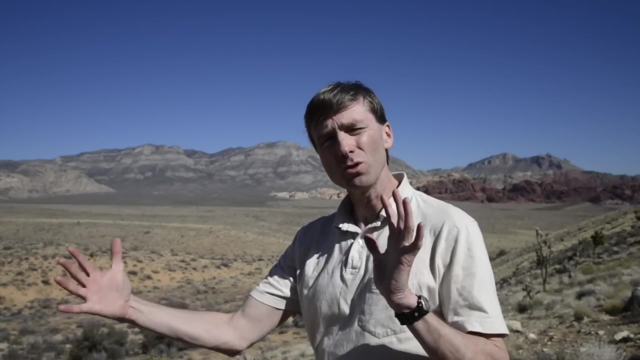 the reverse faults developed first and which developed last and how they form and change orientation during the process shortening. so in this case we have sort of a normal in sequence thrusting history and the result is a very nice imbricate structure. so that's about shortening and the structures that form during shortening of the crust. 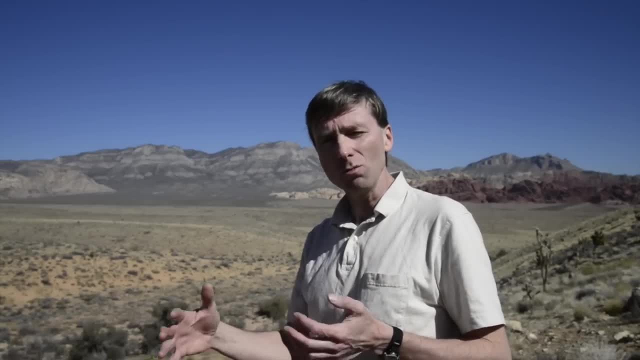 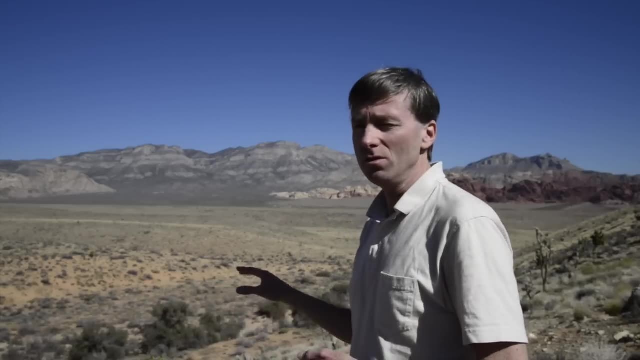 we could also extend the crust and, like i said, we get normal faults, extensional faults and we have to go somewhere else to. well, there are extensional faults here too, but let's go to to a place in utah to show you what an extensional fault looks like. 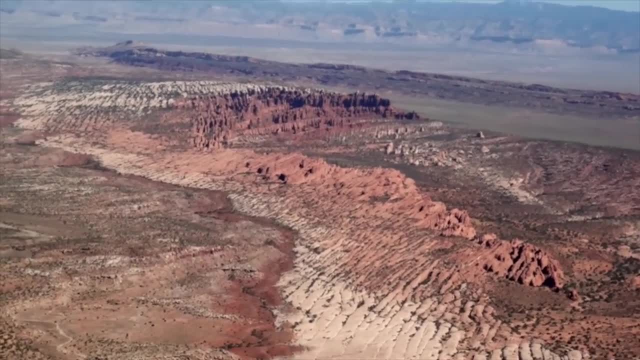 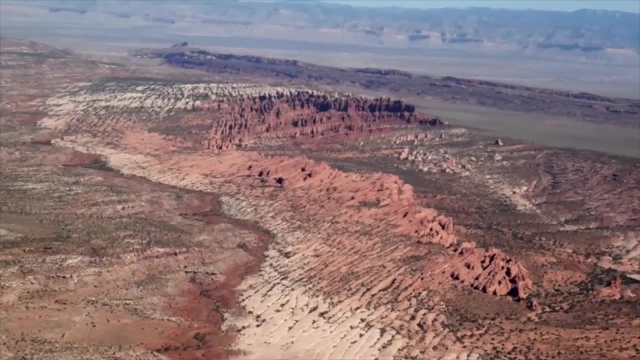 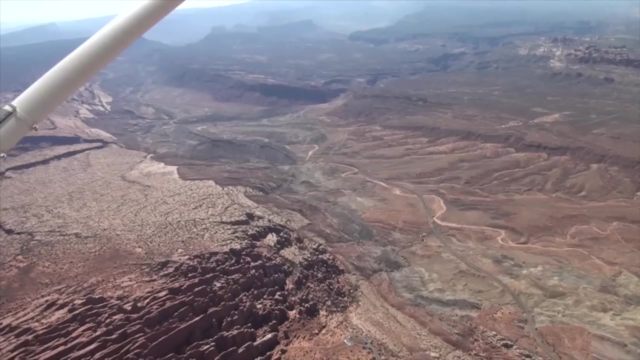 the geology of southern utah is beautifully exposed and right here we're flying over arches national park and we can. we can see sandstones of jurassic age with several sets of fractures. if we go down on the ground, we will see not only fractures but also 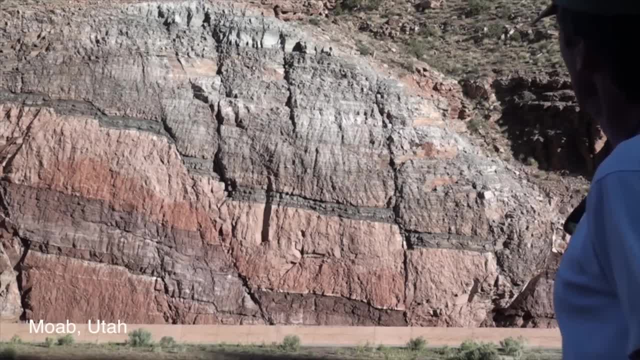 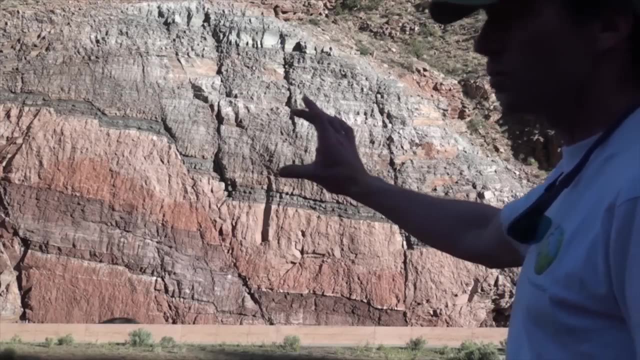 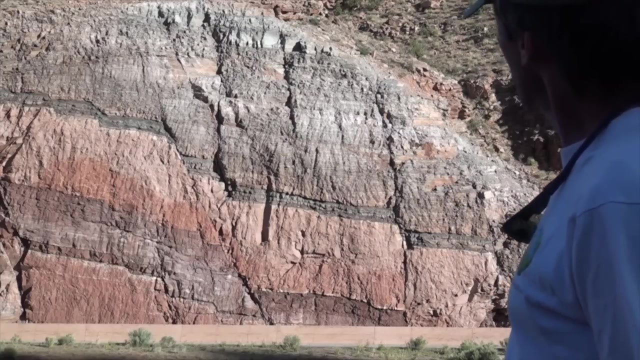 faults. look at those beautiful structures on the other side of the road. those are faults affecting sedimentary layers, sandstones, shales that were once continuous layers and they were affected by these faults in a very interesting way. in this case, we have normal faults. normal faults are extensional structures. that means that at some point in time, 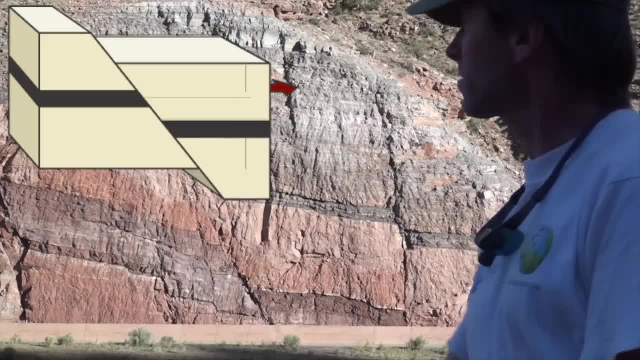 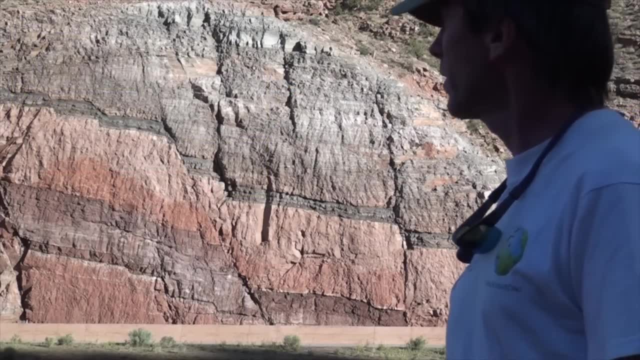 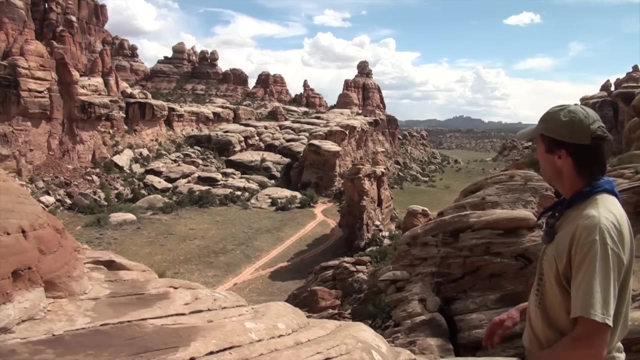 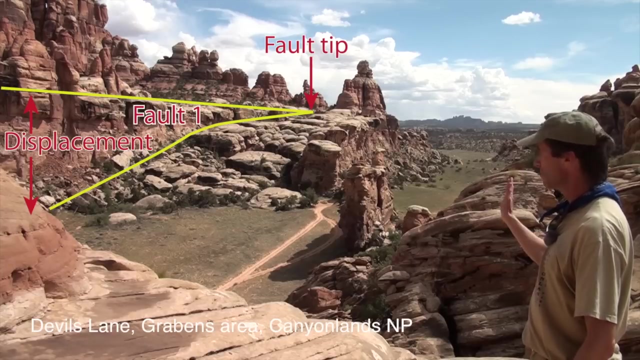 forces were trying to pull these rock layers apart and they partly succeeded and these faults formed. so that's useful information for us astrologists. what happened back in time is a really interesting place where we can see that the displacement on one fault is decreasing. at the same time, another fault picks up the displacement, so the displacement 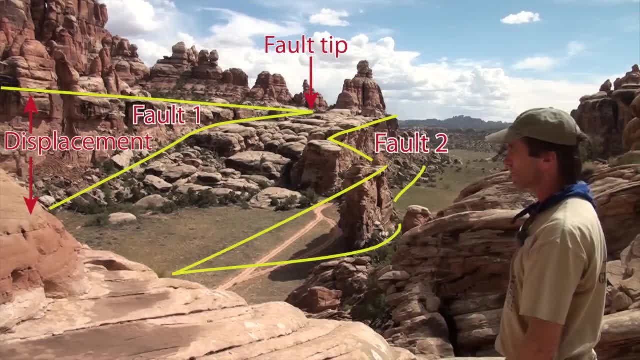 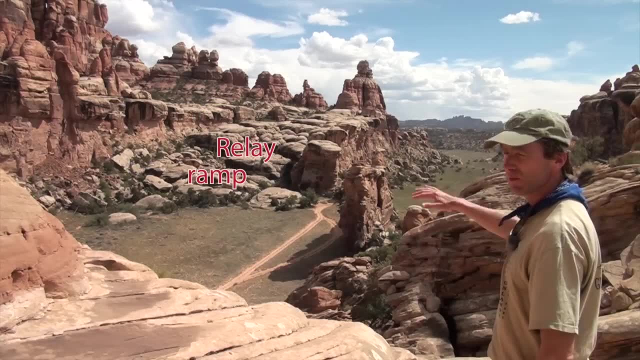 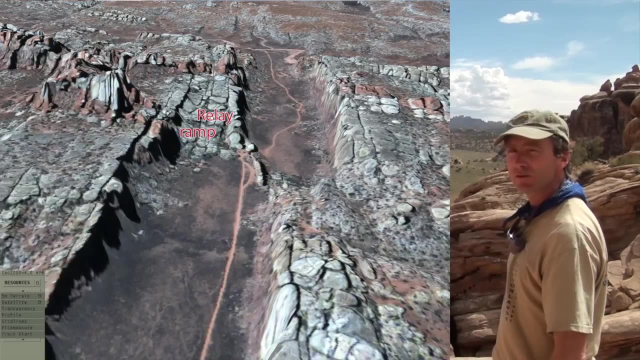 is basically relayed from one fault to to another and we have a relay zone and in between these two faults there's what's called a relay ramp where layers have been folded and- and in this particular case we actually have two sets of relay structures and we have actually what's called a graben stepover structure where one graben dies out. 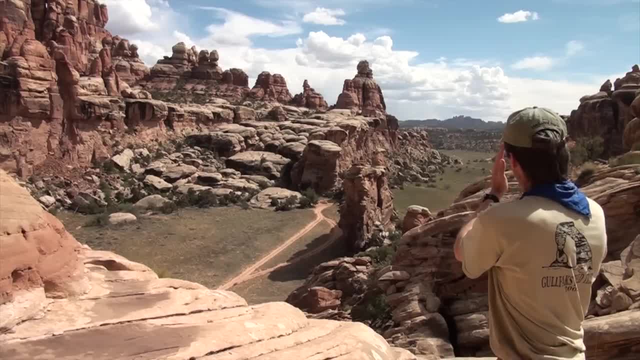 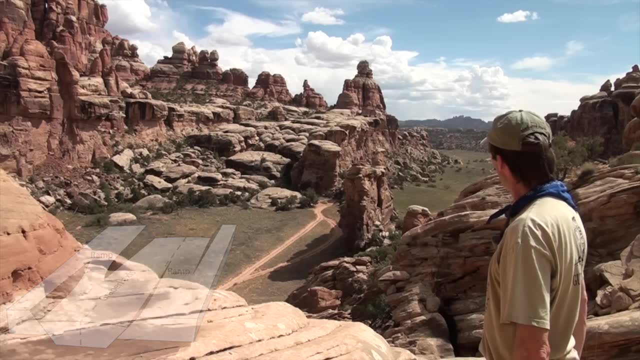 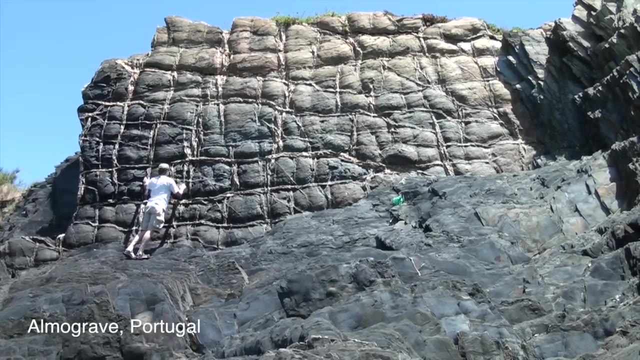 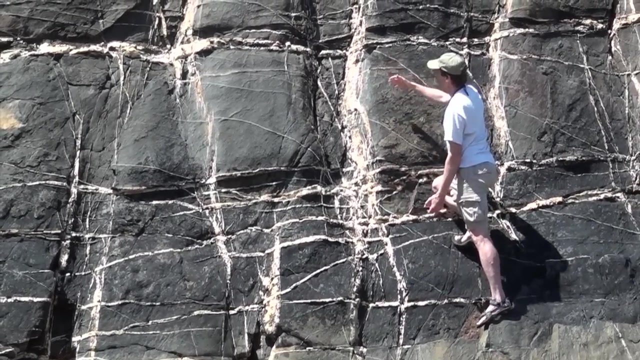 and another one continues, both being parallel with an offset. In some cases we have stretching in two directions, like in these turbidites in Portugal, where we have quartz veins, a vertical set of quartz veins and a horizontal set of quartz veins, and together these imply vertical and horizontal stretching. So we have a structure that 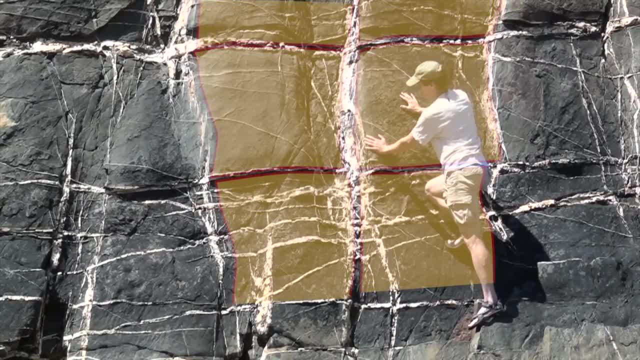 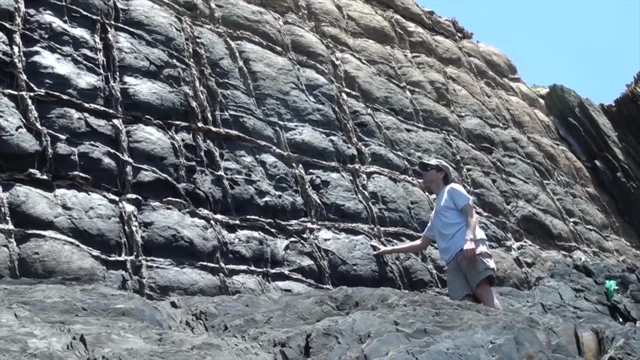 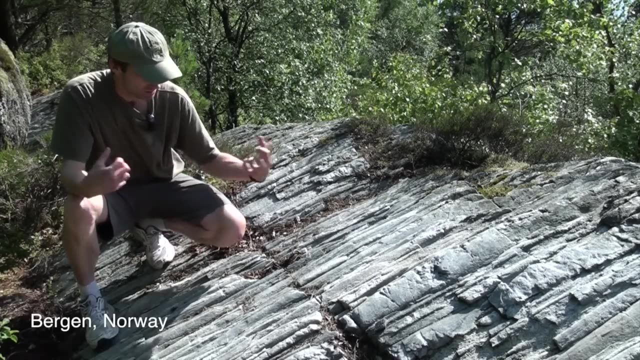 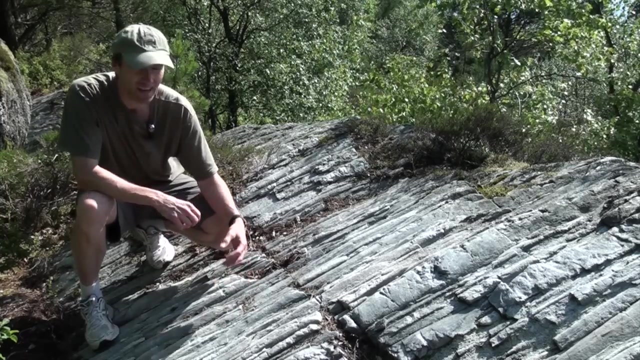 is called chocolate boudinage structure and the strain field that it implies is flattening strain. So we've seen sandstones and sediments being deformed, forming faults and fractures. In this case the sediment has not fractured. It has deformed in a very different way These pebbles and cobbles that were once part. 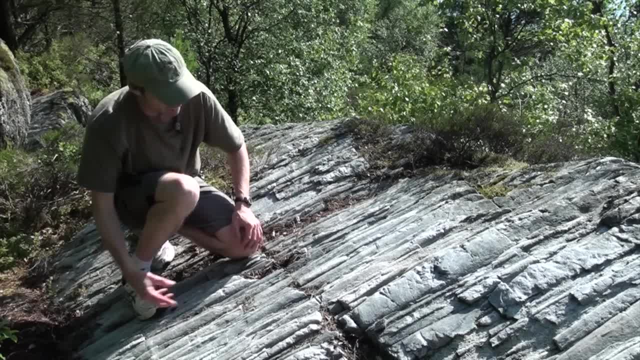 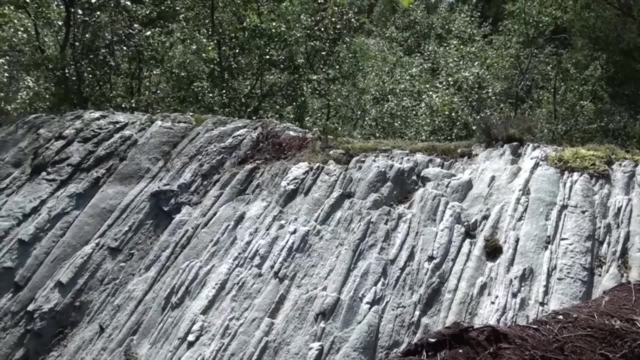 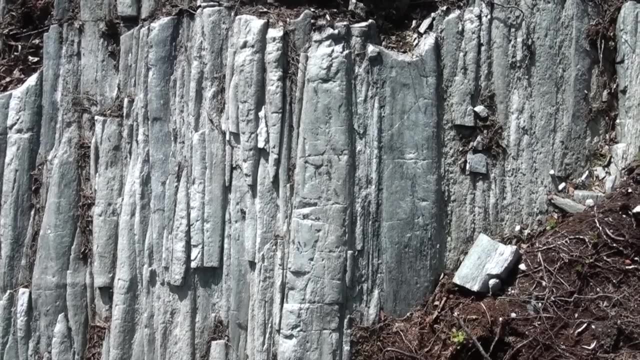 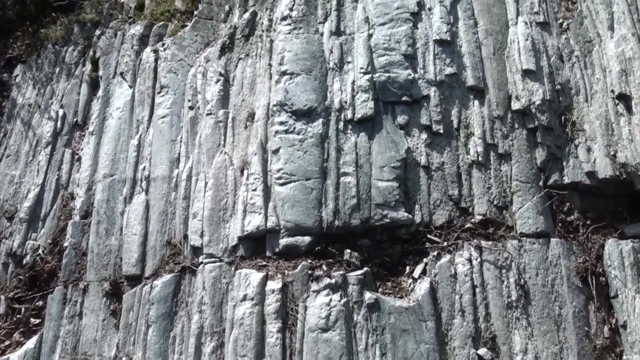 of a conglomerate has now been stretched out into these very elongated objects, almost cigar or walking stick shaped geometries. So the rock, in this case, behaved like a very soft material And we're talking ductile or plastic deformation, And this happens deeper down in the crust. 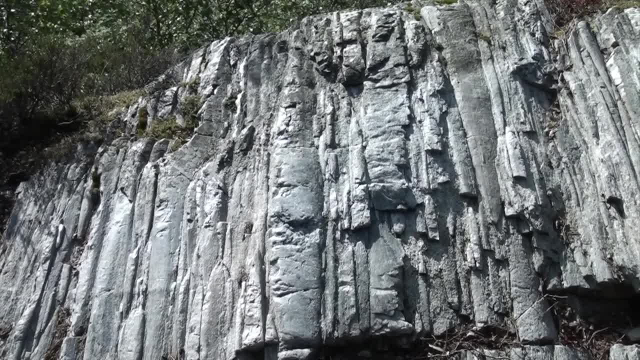 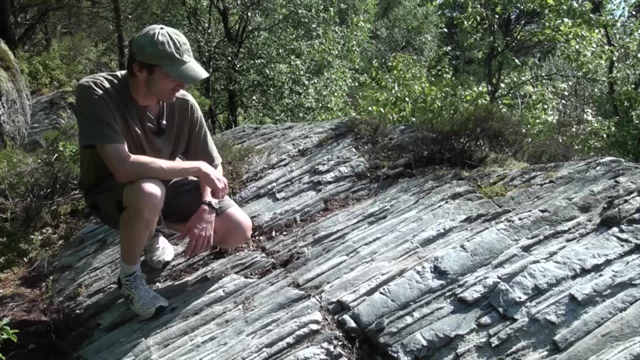 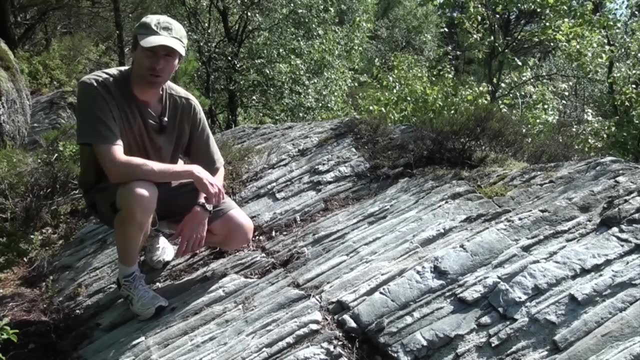 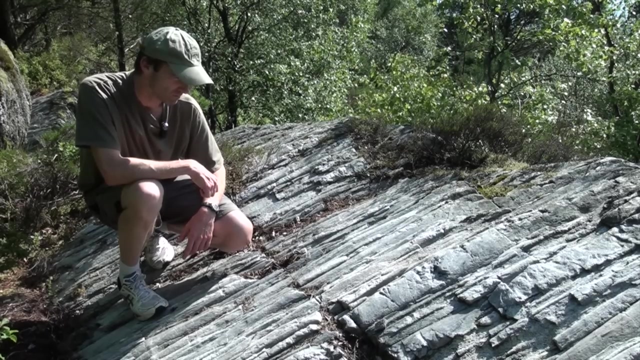 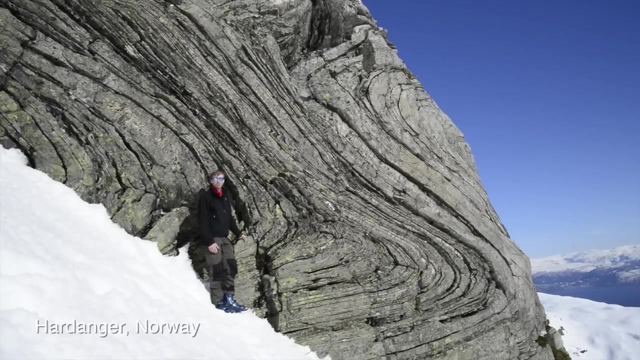 where the temperature gets high and rocks start to flow. So a very different expression of deformation. Temperature, crustal depth are very important parameters when it comes to the way that rocks respond to forces and stresses in the crust. So we'll keep going. 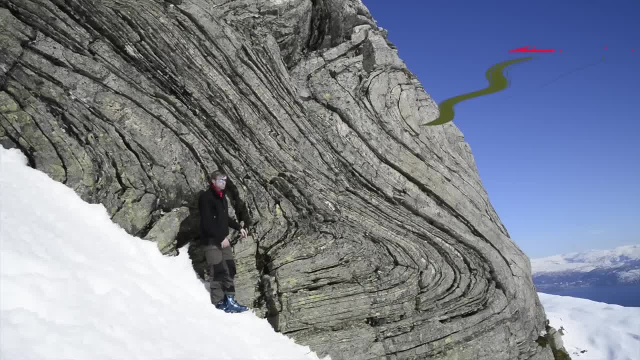 So here's another example: rocks that have deformed in the ductile fashion. We're looking at gneisses and we're looking at a fairly nice fold. So to fold a gneiss like this we need temperatures of, say, 350 degrees or more. So we know that we've been 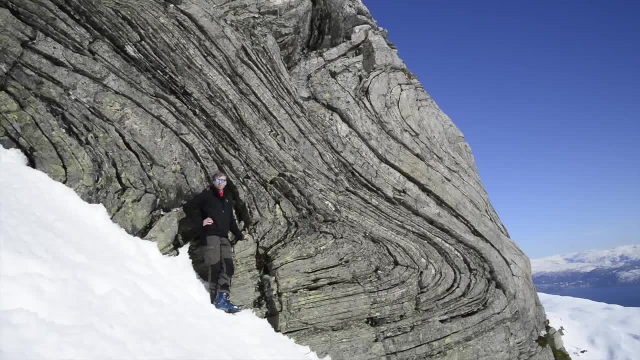 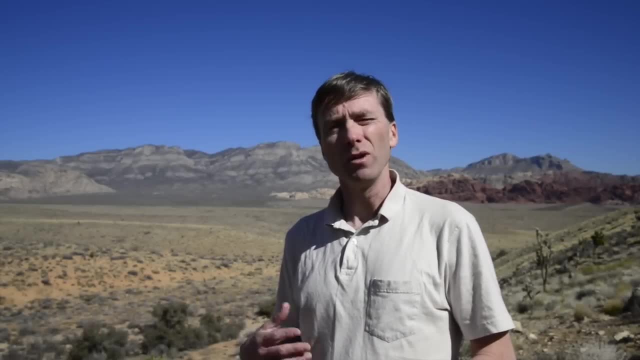 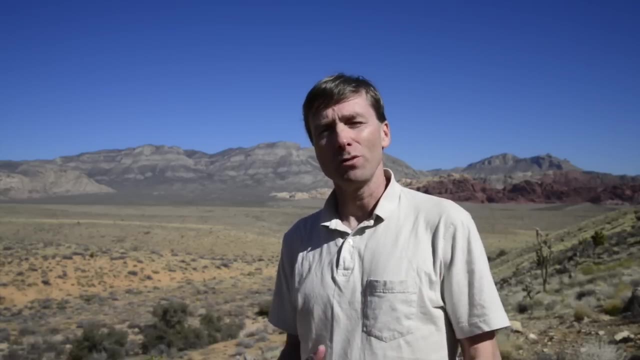 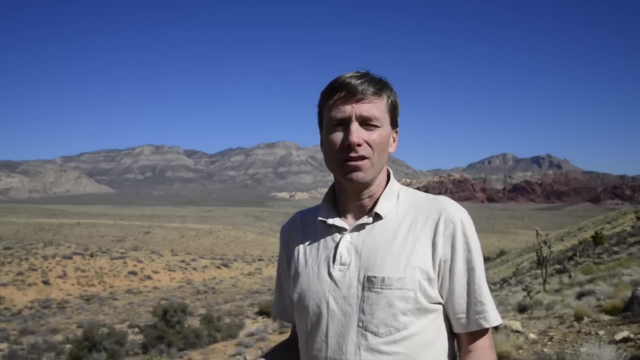 So we're in the ductile regime. The aim is to understand the history behind the formation of these structures, the processes involved and to understand what was going on in the past, at the time when the structures formed many possibilities. We talk about tectonics. 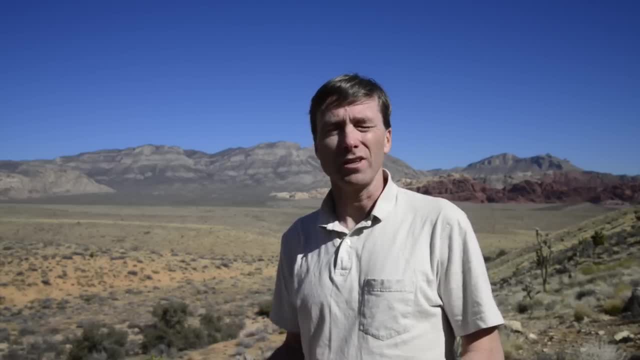 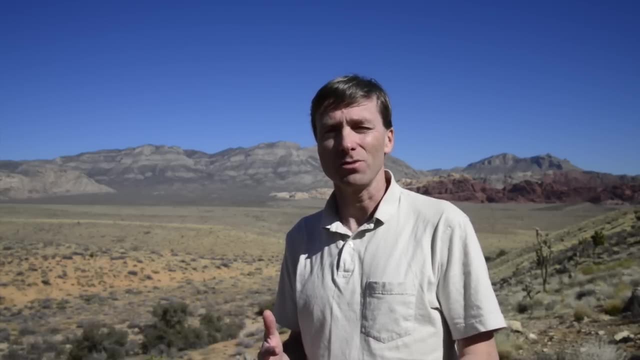 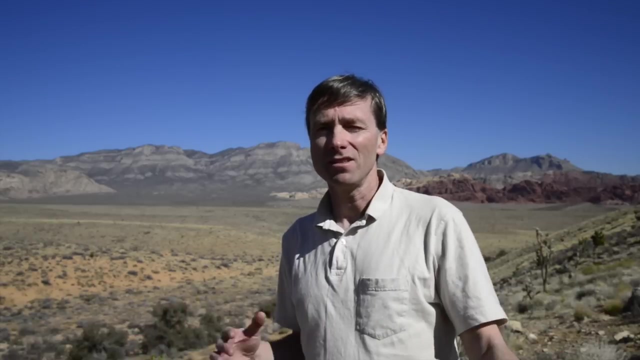 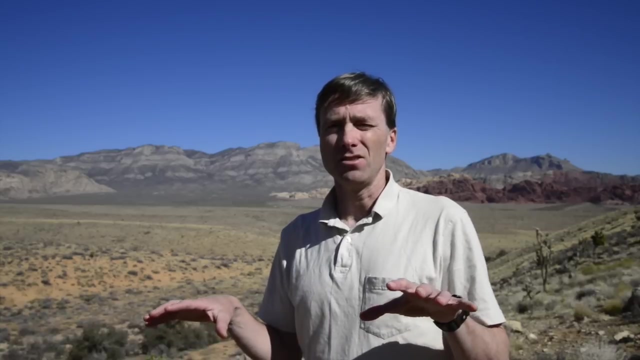 So structural geology and tectonics are sort of walking hand in hand. pretty much all the time We use structure to understand the tectonic history. So tectonics is more about large-scale motions, oftentimes plate motions, And when plates move they create structures. 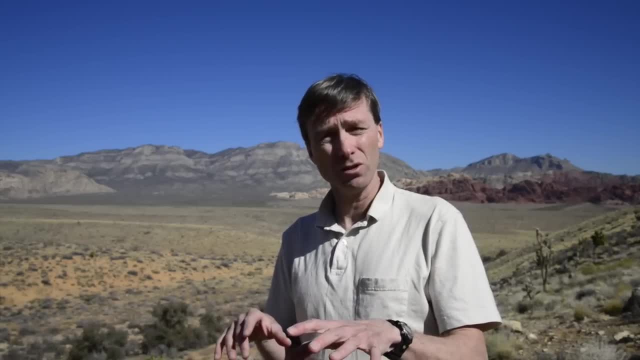 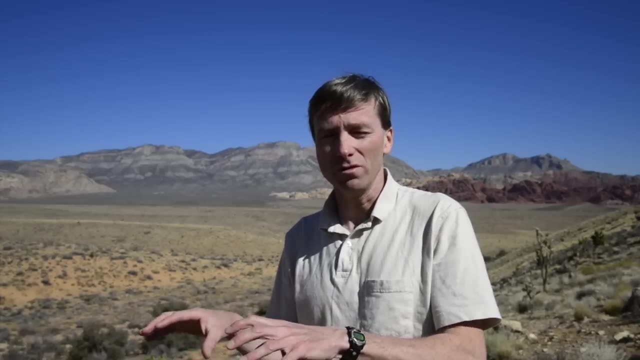 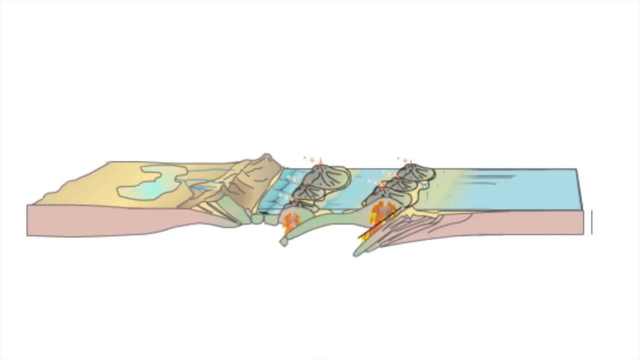 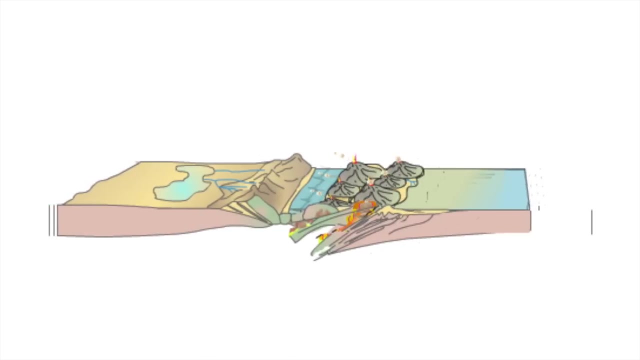 So if we know the plate motions- we could- We would expect certain types of structures to form depending on how the plates move. I mean, if plates converge, you would expect to find what's called reverse faults: thrusts, folds of large-scale folds and mountain chains, orogenic belts.